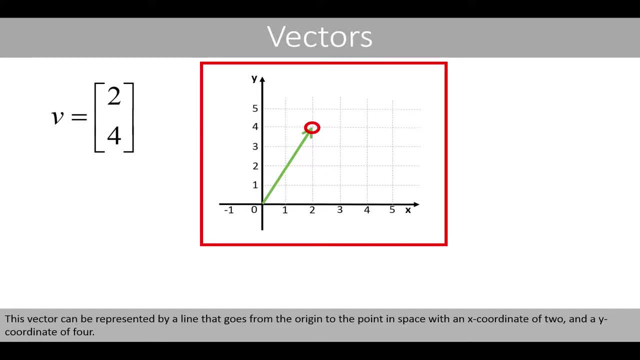 Let's consider another vector. This vector can be represented by a line that goes from the origin to the point in space, with an x-coordinate of 2 and a y-coordinate of 4.. The length of this vector is the square root of 20,. 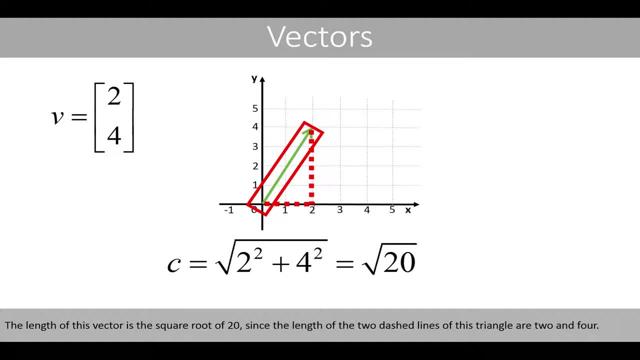 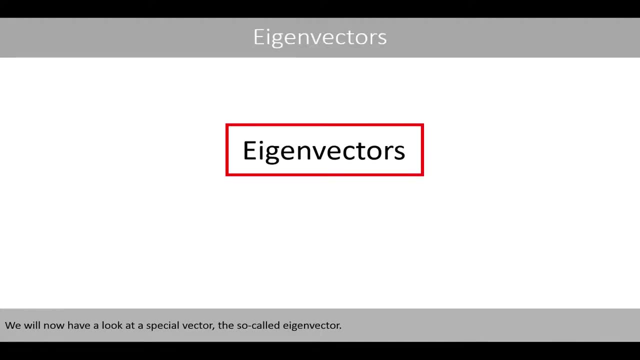 since the length of the two dashed lines of this triangle are 2 and 4.. We'll now have a look at a special vector, the so-called eigenvector. An eigenvector v is a non-linear vector. It's a non-zero vector that satisfies the following equation: 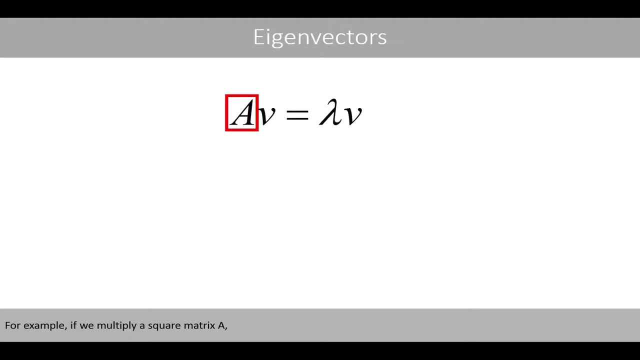 For example, if you multiply a square matrix A by a column, vector v, and if you get a new vector that is equal to a number times the old vector, then vector v is called an eigenvector of matrix A. One can think of this as if you multiply matrix A by vector v. 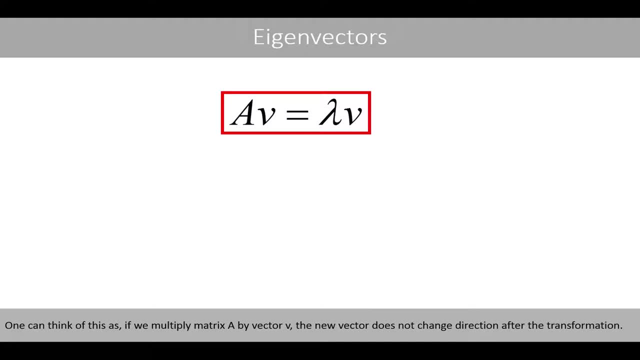 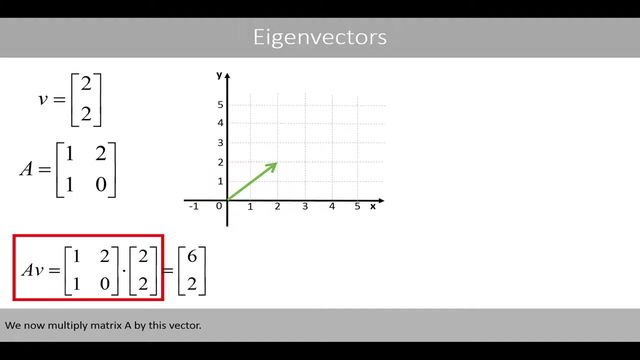 the new vector does not change direction after the transformation. Let's test if the following vector is an eigenvector of matrix A. The vector can be represented in space like this: We now multiply matrix A by this vector. We see that we have got a new vector. 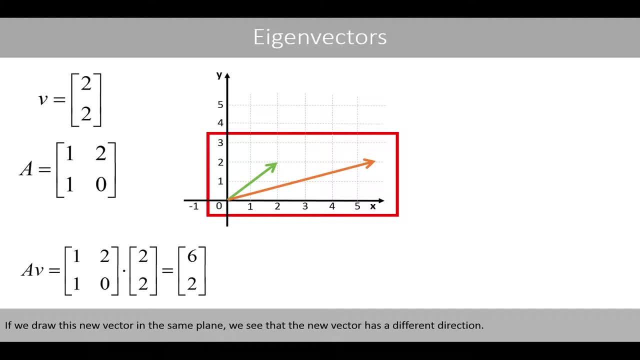 If we draw this new vector in the same plane, we see that the new vector has a different direction. Since this vector changes its direction when multiplied with matrix A, we can conclude that this vector is not an eigenvector of matrix A. Let's see if the following vector is an eigenvector of the same matrix: 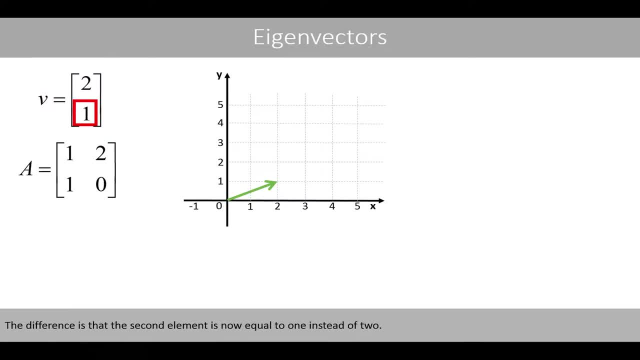 The difference is that the second element is now equal to 1 instead of 2.. If we multiply matrix A by this vector, we get a new vector. If we draw this vector in the same plane, we see that the new vector is not an eigenvector of matrix A. 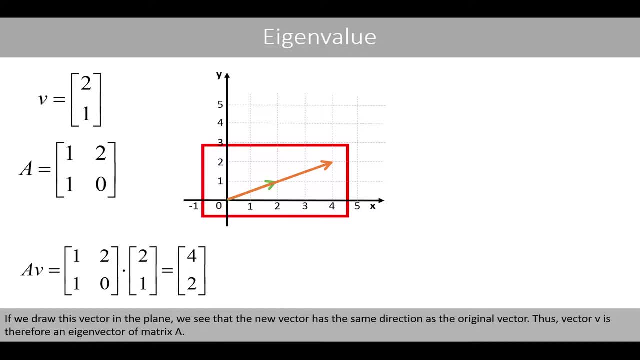 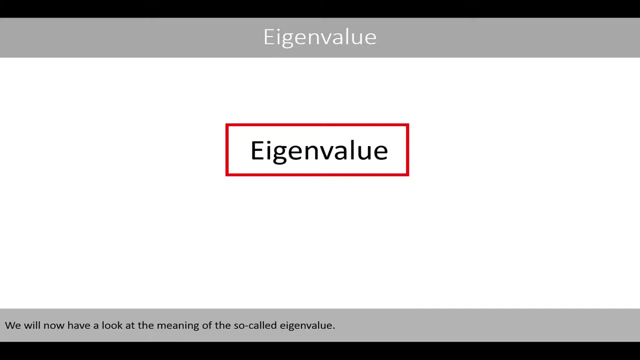 We see that the new vector has the same direction as the original vector. Thus, vector v is therefore an eigenvector of matrix A. We'll now have a look at the meaning of the so-called eigenvalue. The eigenvalue tells us how much the eigenvector changes in size when multiplied with the matrix. 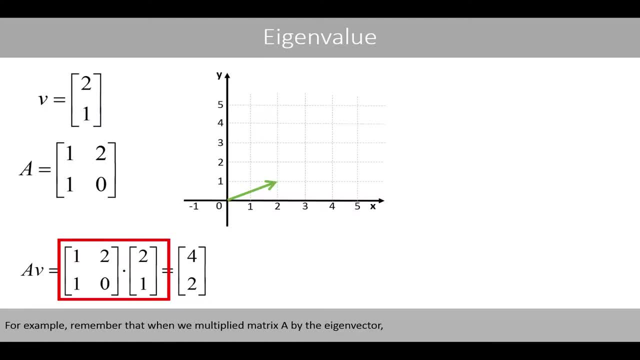 For example, remember that when we multiplied matrix A by origin, we got a new vector of this vector 2 times the original vector. The associated eigenvalue to the eigenvector is therefore equal to 2.. The eigenvalue is usually denoted by lambda. 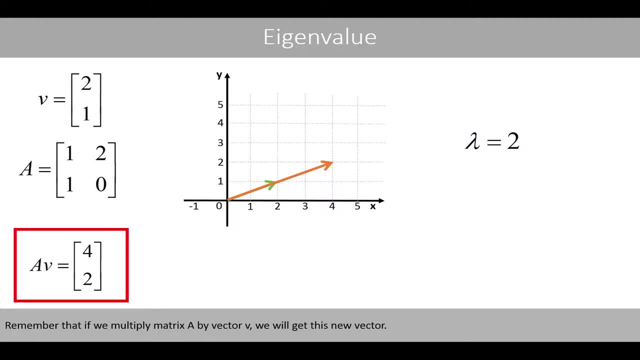 Remember, in terms of the result, that 6 times the original vector is a relation of 2, for many Auto viergon vectors, and 0 to시에ize vectors, which also has a depreciation value of 1.. The vector v is therefore an eigenvector of matrix A. 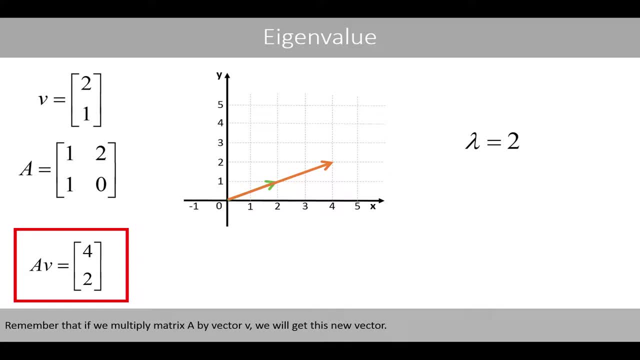 Remember that if we multiply matrix A by vector v, we will get this new vector. This new vector can be written like this, where 2 is the eigenvalue and this is our original vector v. Thus, if we multiply matrix A by the eigenvector, we will get a new vector. 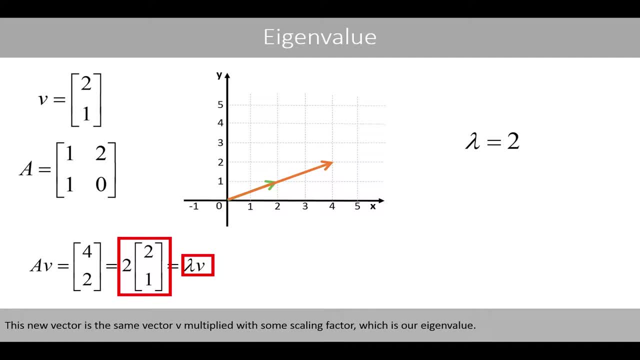 This new vector is the same vector v multiplied with some scaling vector, which is our eigenvalue. We can therefore conclude that an eigenvector of matrix A results in a new vector that has the same direction as the original vector, but which might be either longer or shorter than the original vector. 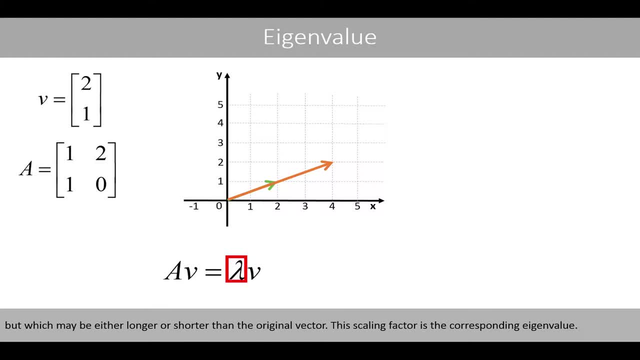 This scaling vector is the corresponding eigenvalue. Note that the eigenvalue can even be negative, which means that the direction of the new vector is reversed, but still on the same line. For example, in this case the eigenvalue is equal to negative 1, because the new vector 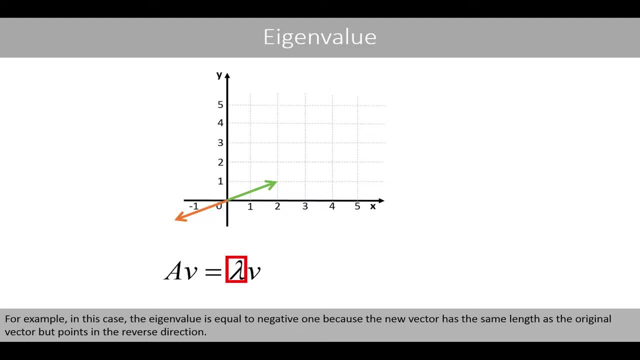 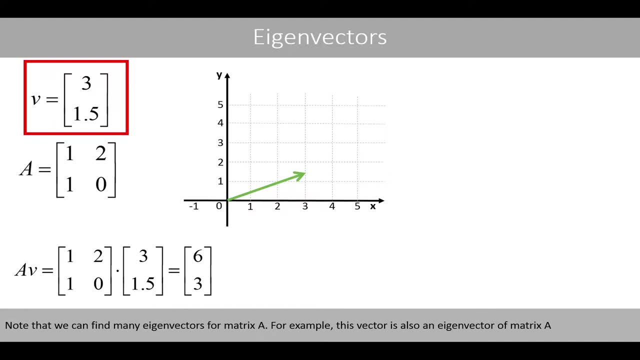 has the same length as the original vector but points in the reverse direction. Note that we can find many eigenvectors. for matrix A, For example, this vector is also an eigenvector of matrix A. This vector is equal to negative 1, because the new vector has the same length as the. 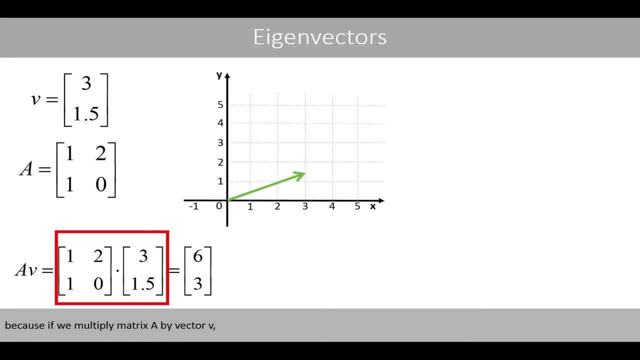 original vector but points in the reverse direction. matrix A: by vector V We get a new vector with the same direction that is twice as long as the original vector. Note that although we have found a new eigenvector, the corresponding eigenvalue does not change. We see that the eigenvalue is still 2.. Also the new vector: 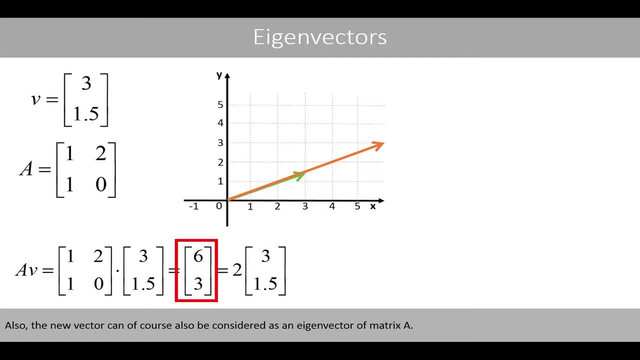 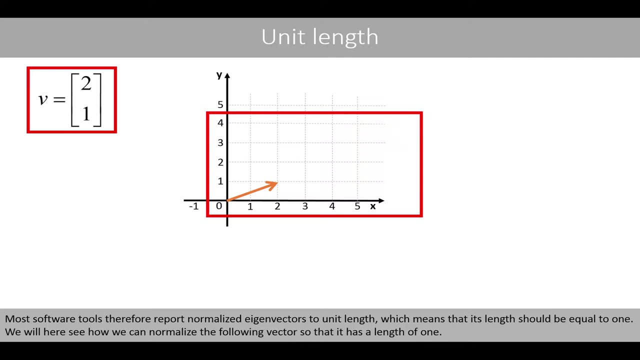 can of course also be considered as an eigenvector of matrix A. All vectors with the same direction are actually eigenvectors of matrix A. Most software tools therefore report normalized eigenvectors to unit lengths. We will here see how we can normalize the following vector so that it has a length of: 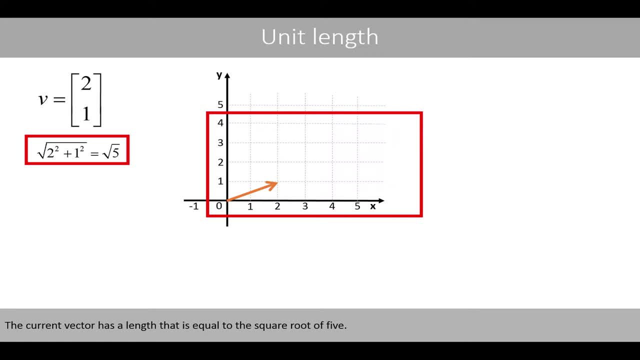 1. The current vector has a length that is equal to the square root of 5.. Let's square both sides. If we divide both sides by 5, the right hand side will be equal to 1.. We can only formulate to this where we see that if we let a vector go from the origin, 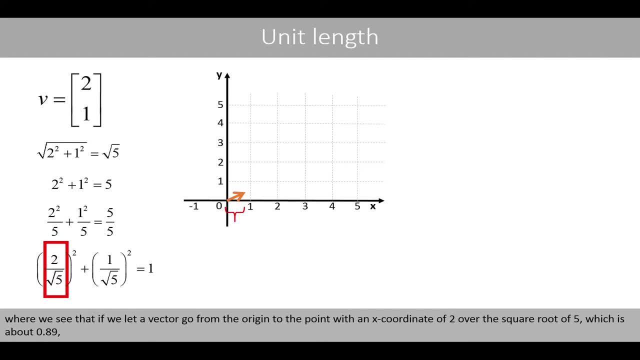 to the point, with an x-coordinate of 2 over the square root of 5,, which is about 0.89, and a y-coordinate of 1 over the square root of 5, which is about 0.45,. the resulting vector: 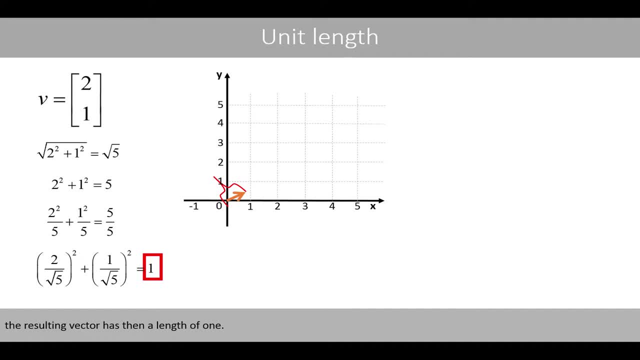 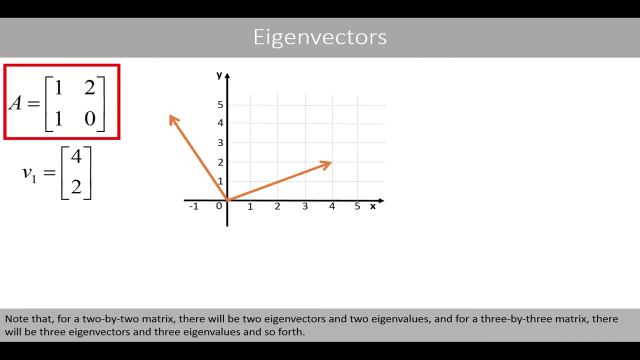 has then a length of 1.. Thus, the following eigenvector is an eigenvector with unit length. If we use the software to find an eigenvector of the following matrix, the software would report the following eigenvector which has a length of 1..